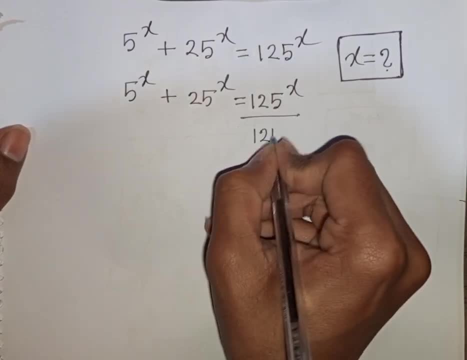 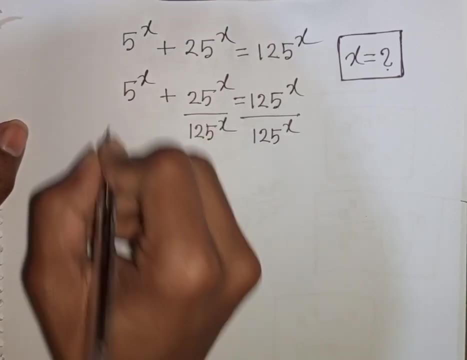 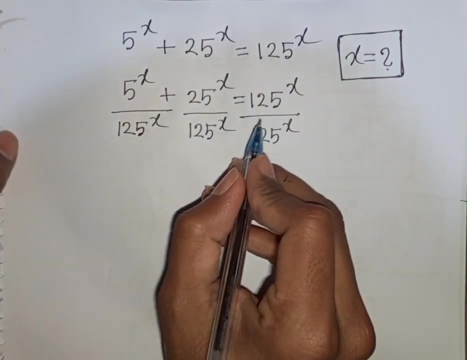 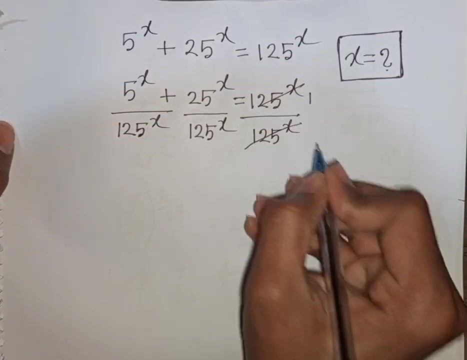 So, divided by 125 power x, divided by 125 power x, divided by 125 power x, Now we see this 125 power x. this 125 power x will be cancelled. So here, on, here, on Now, from here, we see x, x, same power. 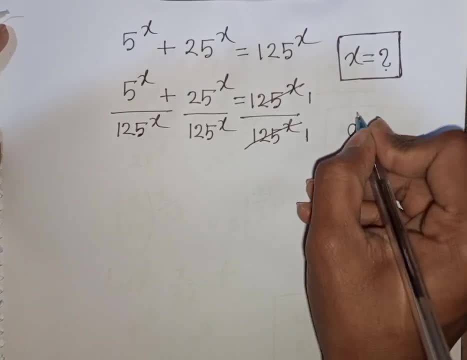 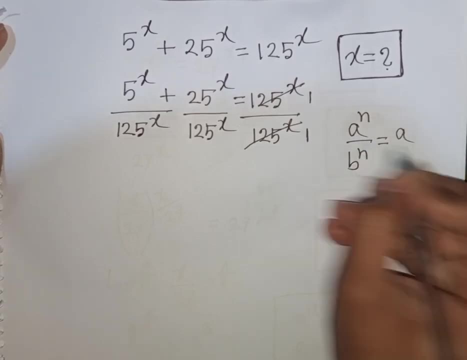 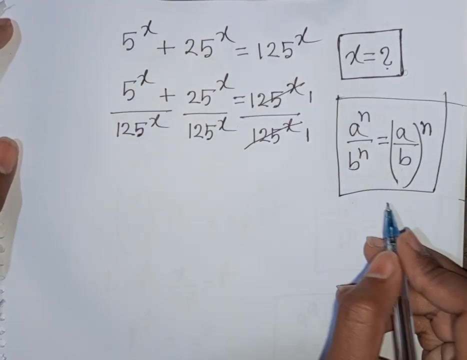 But different base. So remember this formula: A power n over b, power n is equal to a over b. then bracket: common power n. That means n, n, Same power, but different base. So according to this exponential rule we can write here 5 over 100.. 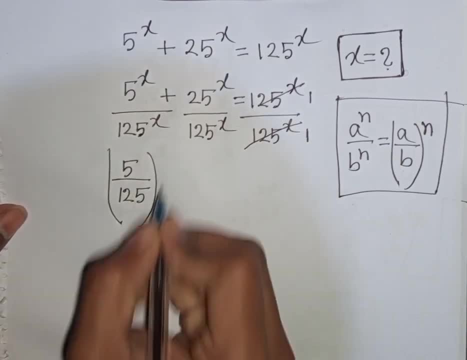 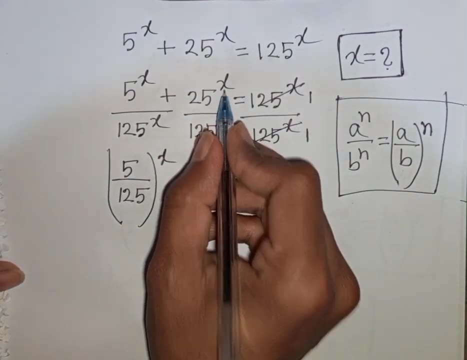 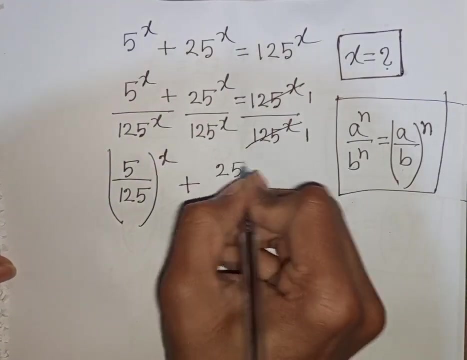 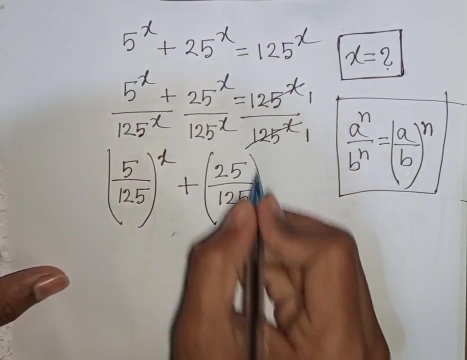 So we have 125 power x plus 125 power x, Then bracket common power x plus again x x. same power but different base. So according to this formula we can write here 25 over 125.. Then bracket common power x is equal to 125. 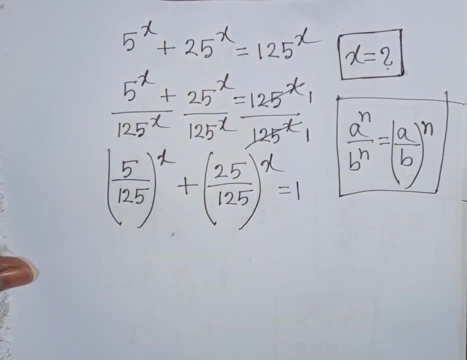 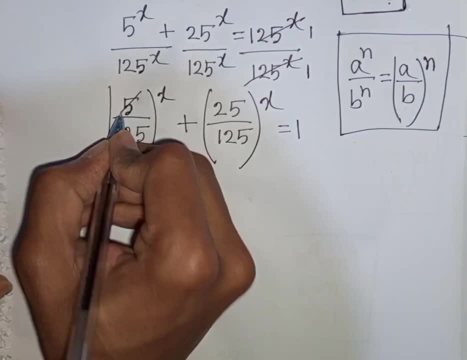 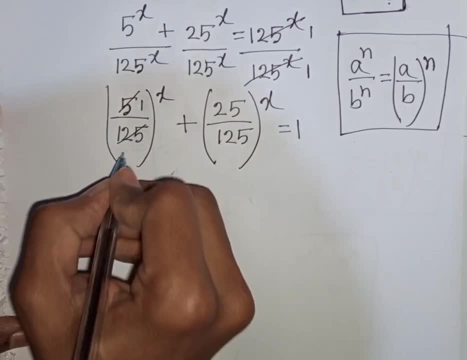 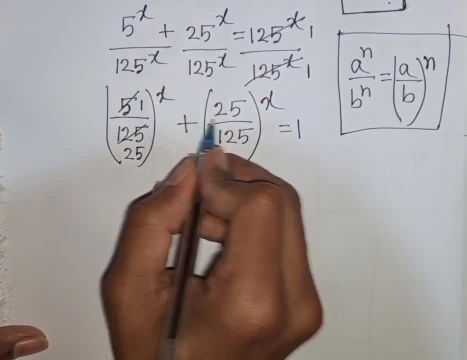 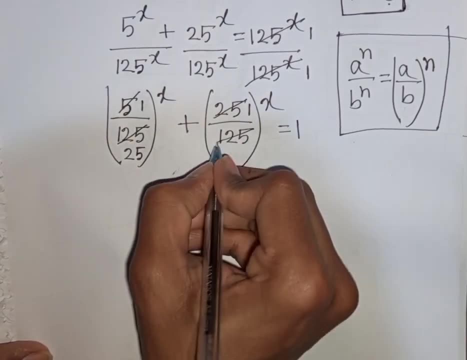 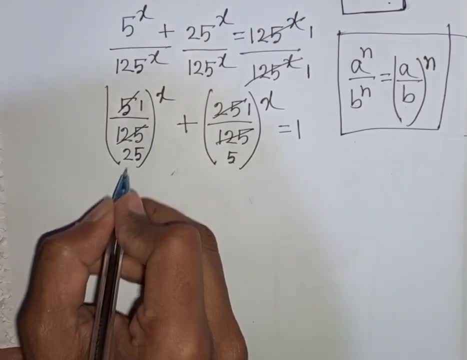 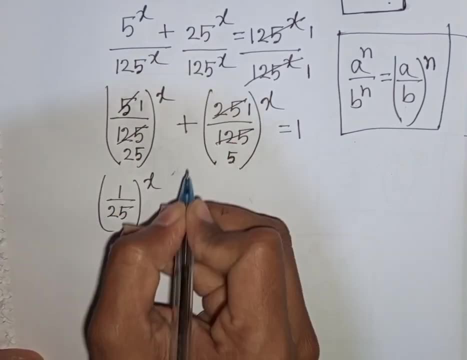 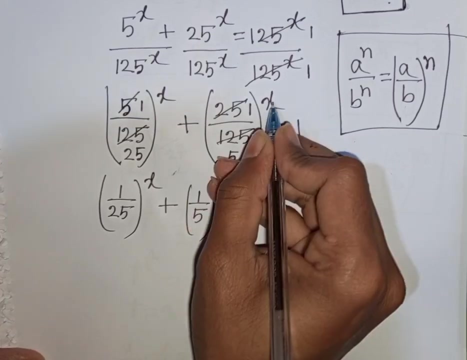 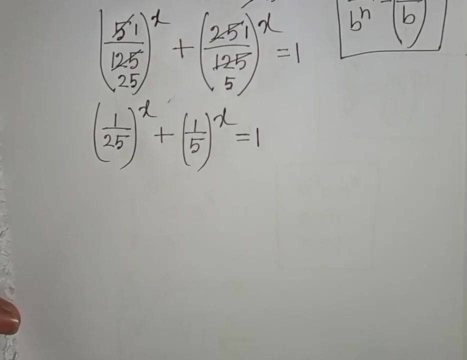 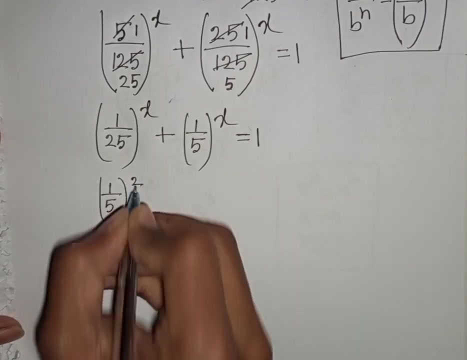 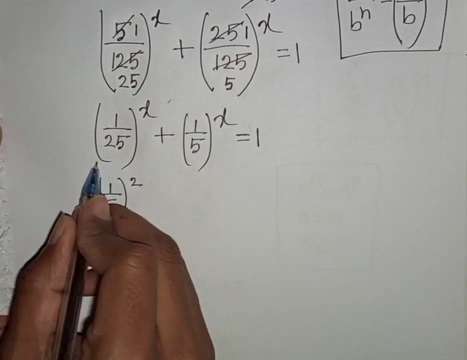 So we have 1 over 25, then bracket power of x plus 1 over 5, then bracket power of x is equal to 1.. Now 1 by 25 can be written as 1 by 5 bracket power, 2. 1 square is same as 1 over 5. square is same as 25.. Then first bracket: 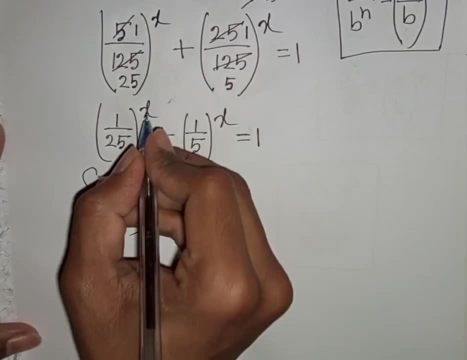 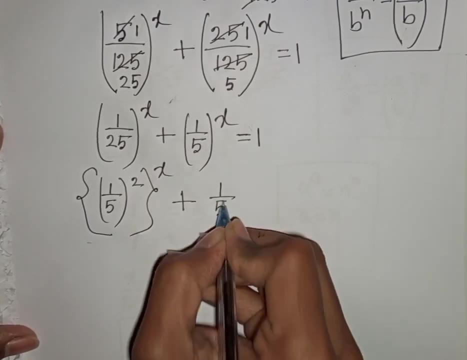 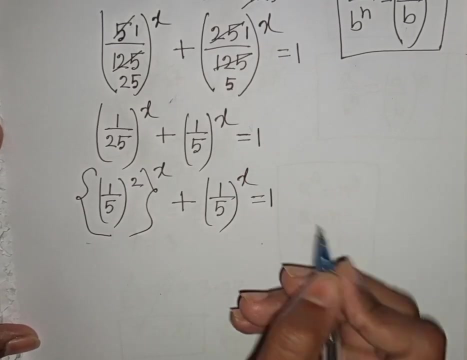 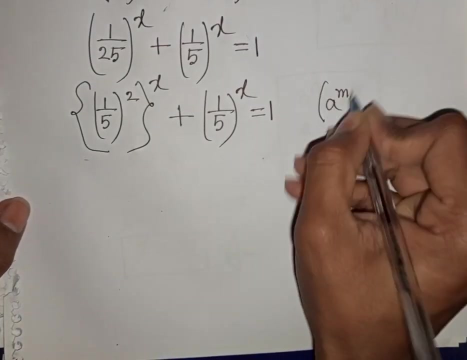 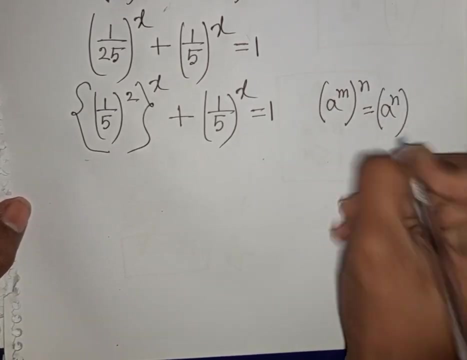 this first bracket can be written as second bracket. then power of x plus 1 by 5 bracket power x is equal to 1.. Now here we can apply this exponential rule that a power m bracket power n is equal to a power n bracket power m. 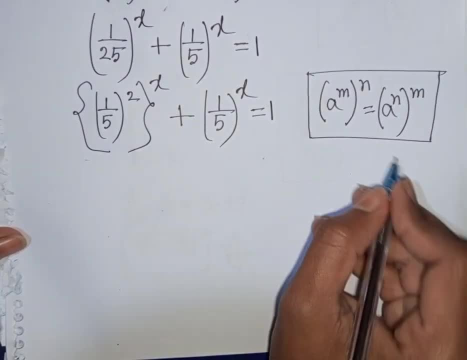 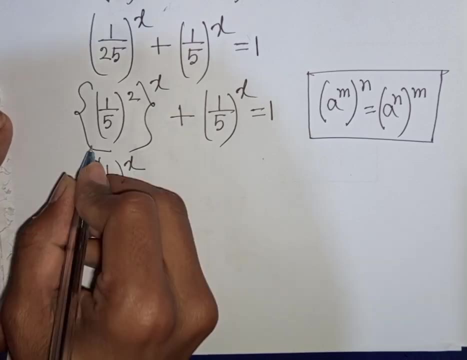 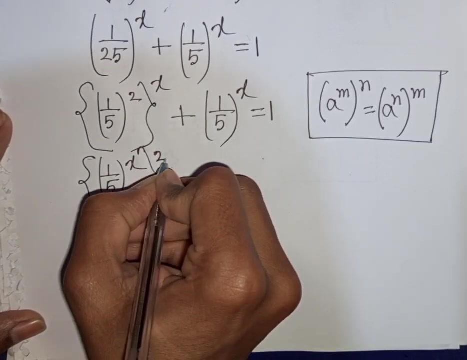 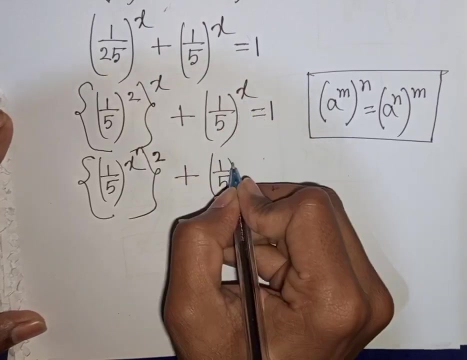 So according to this rule we can write here: 1 by 5 bracket power x, then second bracket, second bracket power of 2, then plus 1 by 5 bracket power x is equal to 1.. Now we see: 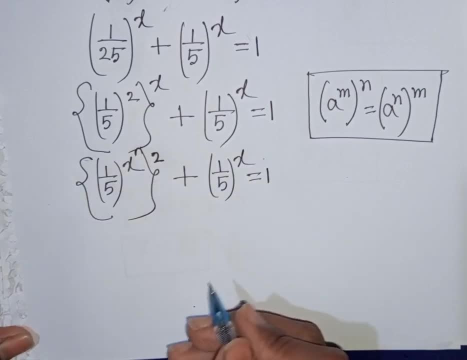 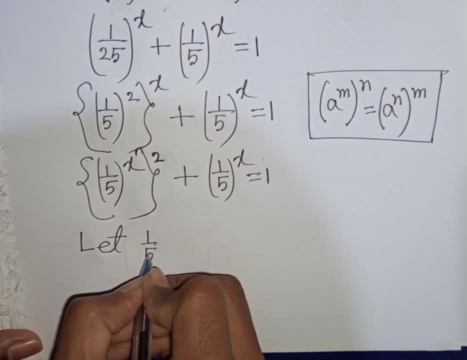 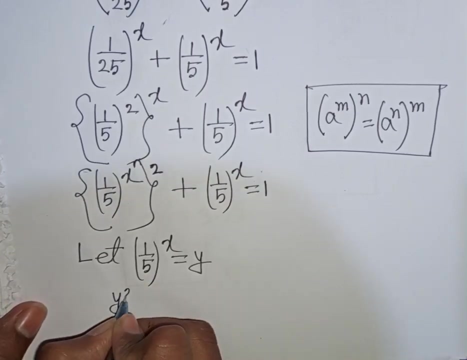 1 by 5 bracket power x. 1 by 5 bracket power x. both terms are the same, So let 1 by 5. bracket power x is substituted by y, So our equation will be y square plus y. 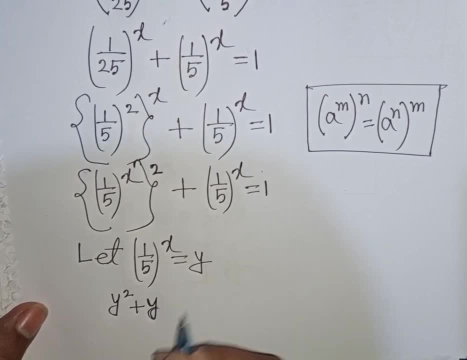 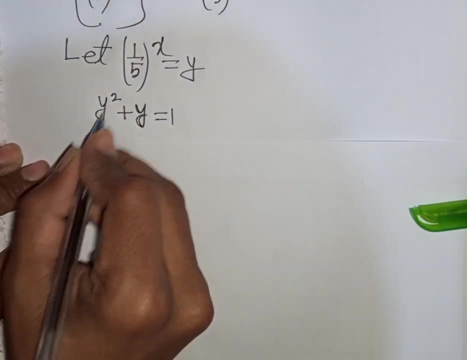 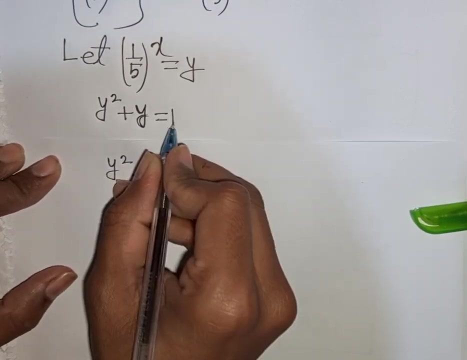 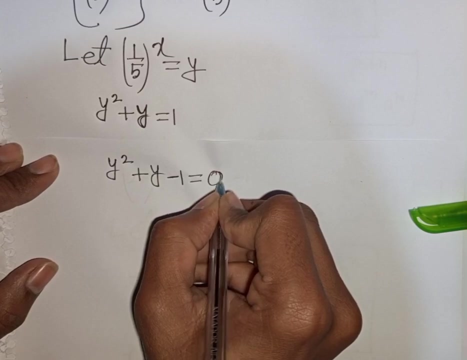 then y square is equal to 1.. Now we can write here: y square plus y, then this plus 1 take to the left side, So this will be minus 1, then a is equal to 0.. Now here you can apply quadratic formula. 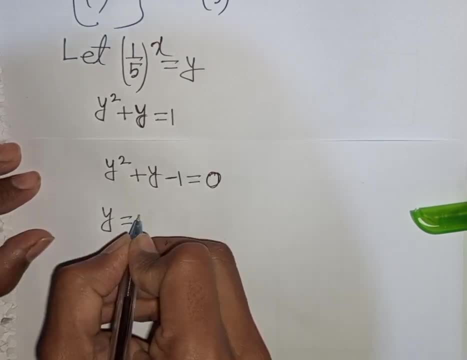 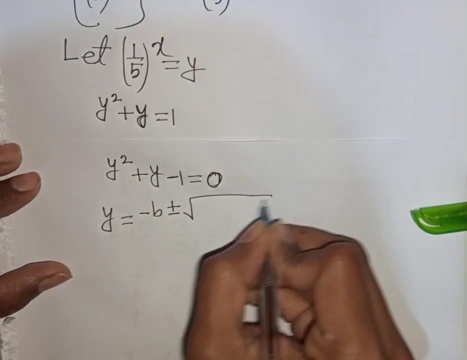 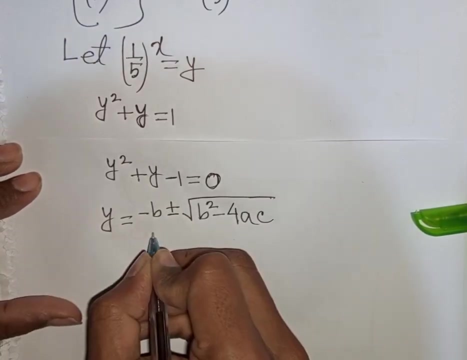 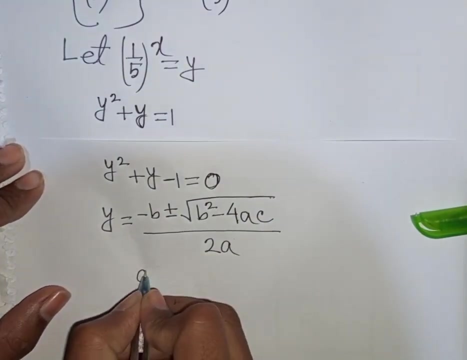 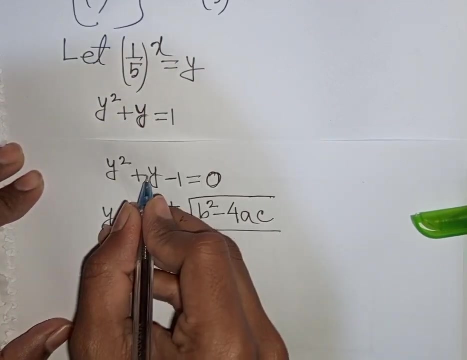 So you can write here: y is equal to minus b, plus or minus a, square root of b, square minus 4ac divided by 2a. So here a will be equal to 1, then b will be equal to 1.. After that c will be equal to 1.. 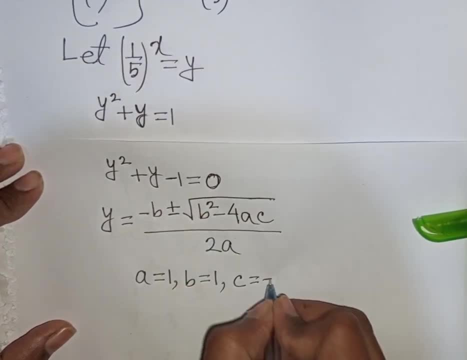 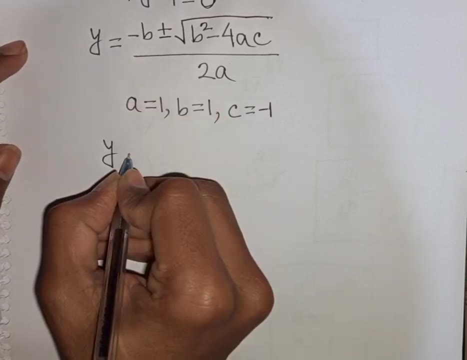 So here you can write here: y is equal to 1, then b will be equal to 1.. Then b will be equal to 1.. equal to minus 1.. Now we can write here: y will be equal to minus b. that means 1,. then. 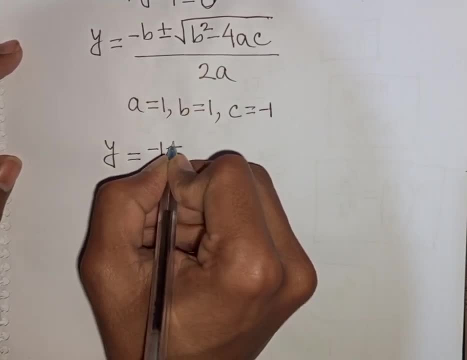 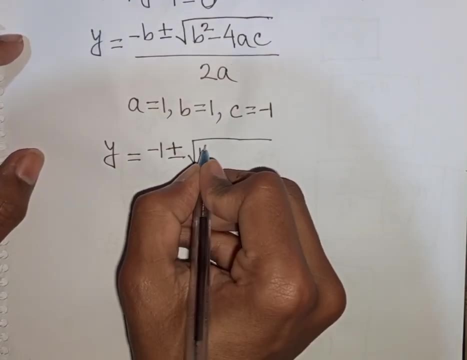 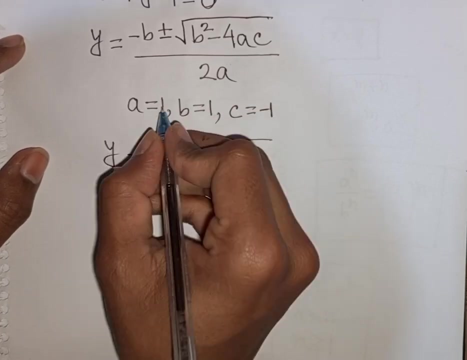 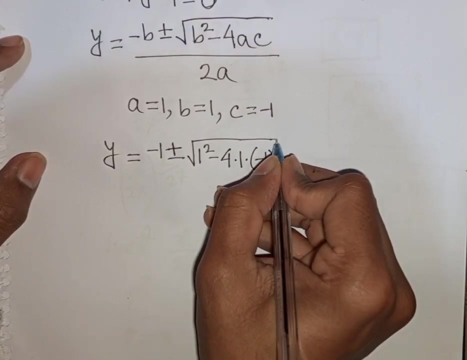 plus or minus square root of b square. that means it will be 1 square minus 4 times a. that means 1 times c, that means negative 1.. So it will be bracket negative 1, then divided by 2 times b square. 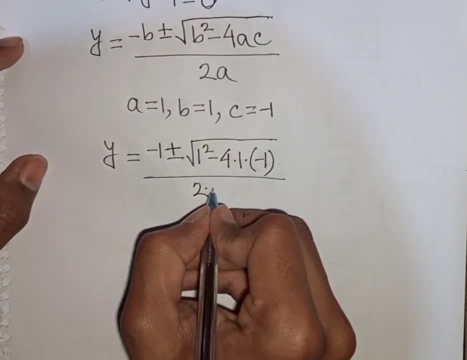 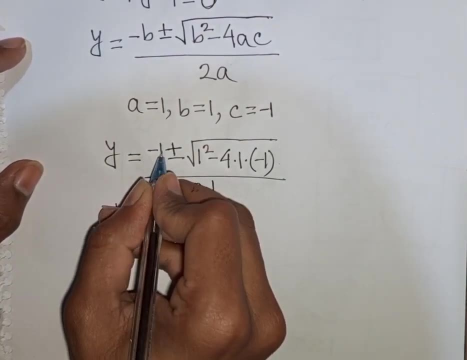 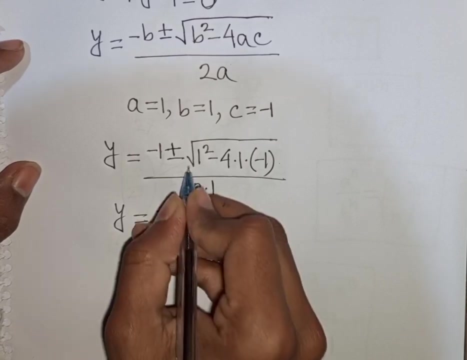 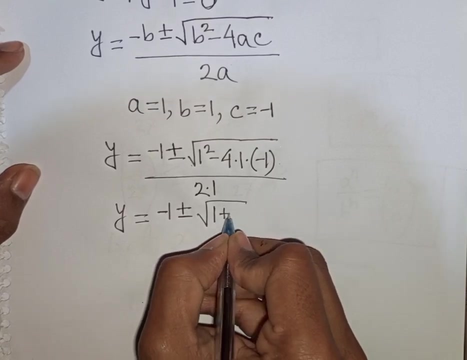 Now we can write here: y is equal to minus 1, plus or minus. square root of 1 square is same as 1, then minus times minus that means it will be plus, then 4 times 1 times 1, that 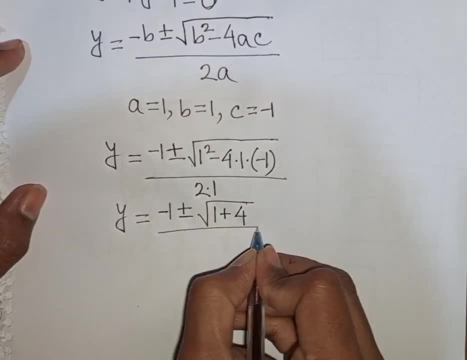 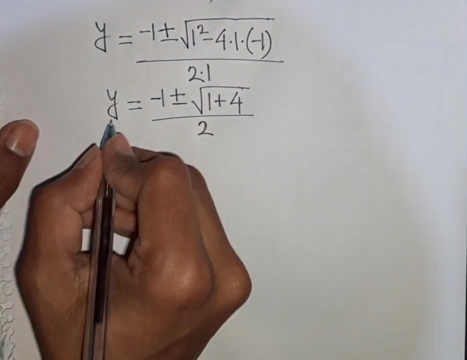 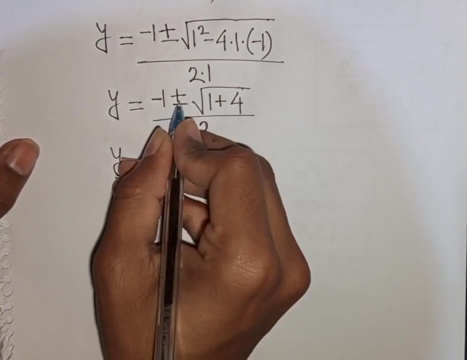 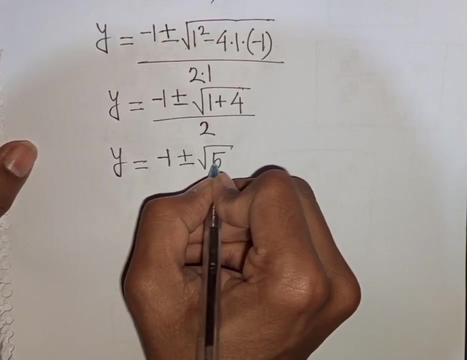 means it will be 4.. Then divided by 2 times 1,, that means 2.. Now we can write here: y is equal to minus 1, minus 1 plus or minus square root of 1 plus 4, that means it will be 5, then divided: 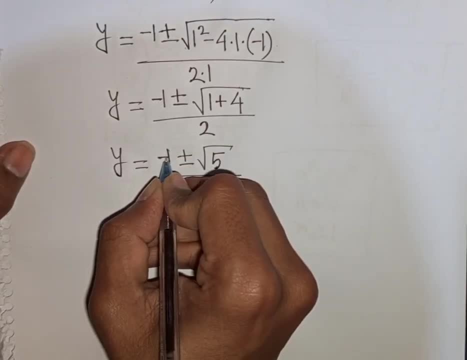 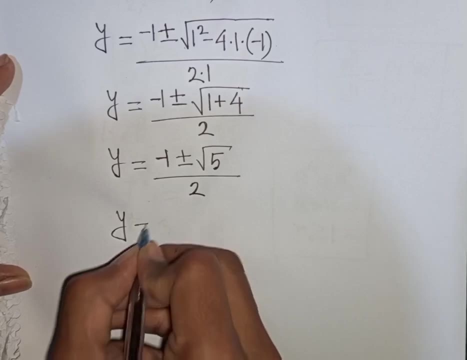 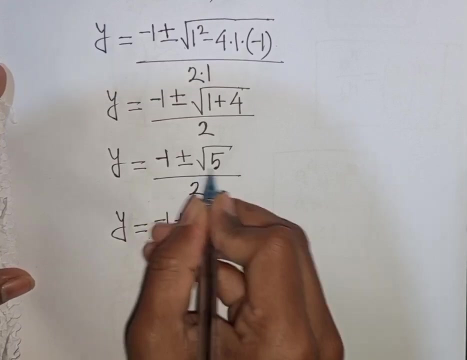 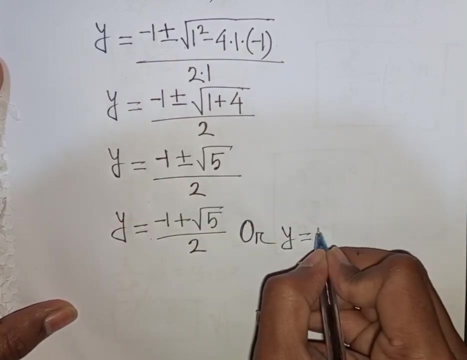 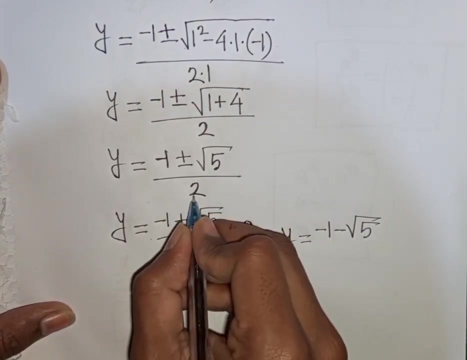 by 2.. Now we see here two cases. so you can write here: y is equal to minus 1 plus square root of 5 divided by 2, or y is equal to minus 1 minus square root of 5 divided by 2.. But remember that y that 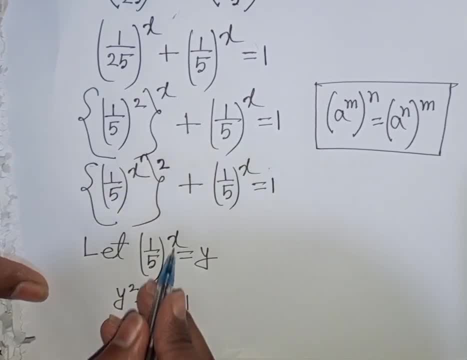 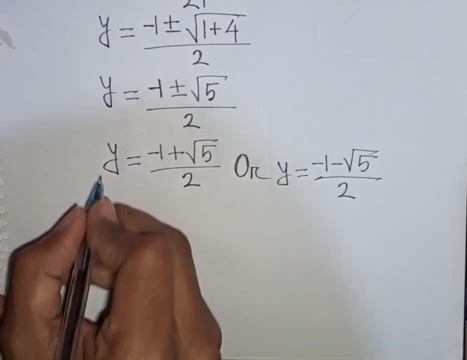 means let 1 by 5 bracket tau x is substituted by y, So y that means it will be 1 by 5 bracket tau x. So y is equal to minus 1 plus square root of 5 divided by 2.. 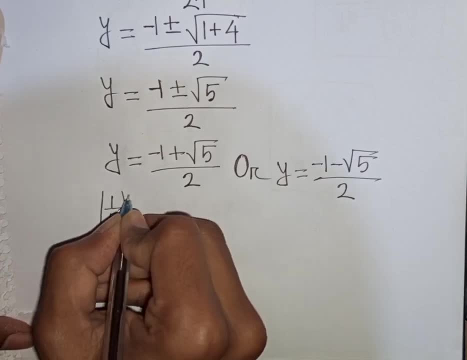 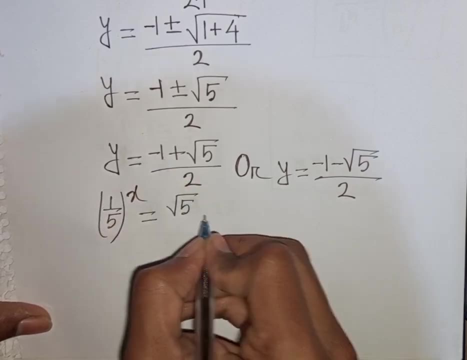 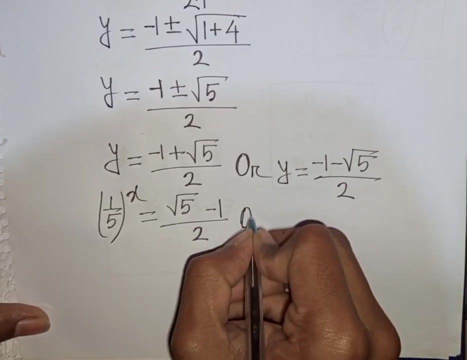 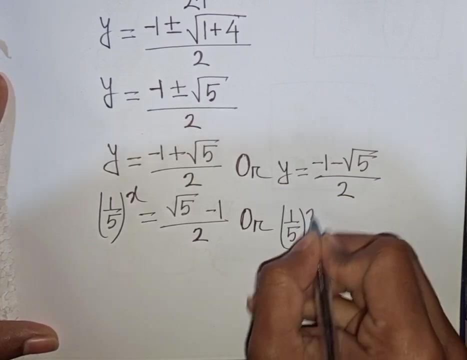 So y, that means 1 by 5, bracket tau x is equal to plus square root of 5,, that means square root of 5, then minus 1 divided by 2. or y, that means 1 by 5, bracket tau x. So. 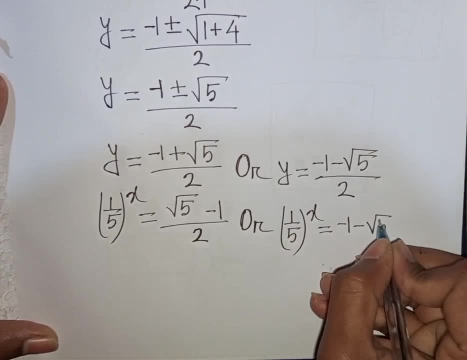 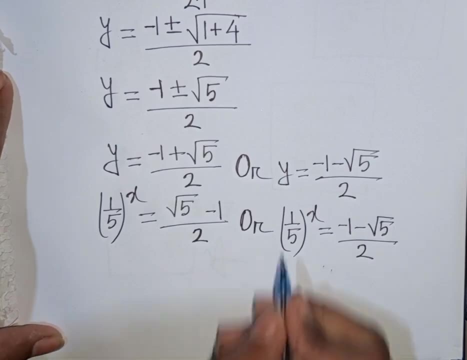 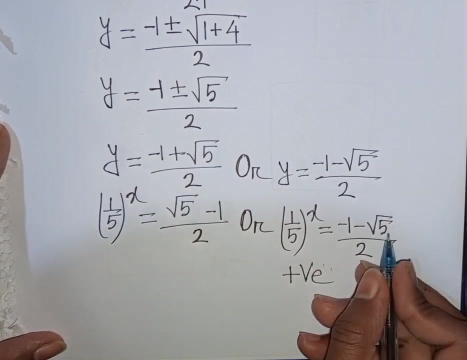 y is equal to minus square root of 5 divided by 2.. Now we see 1 by 5. bracket tau, any number is always positive, but minus 1, minus square root of 5 divided by 2, this is must. 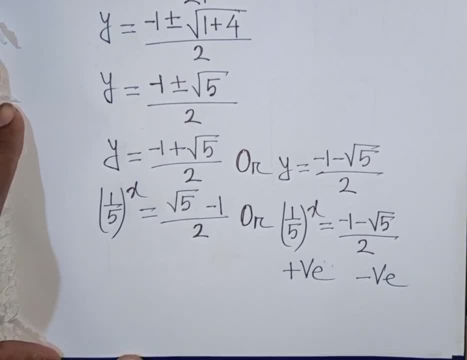 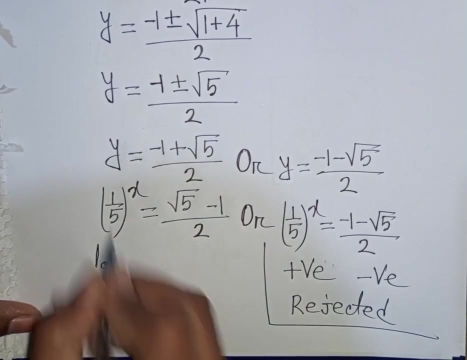 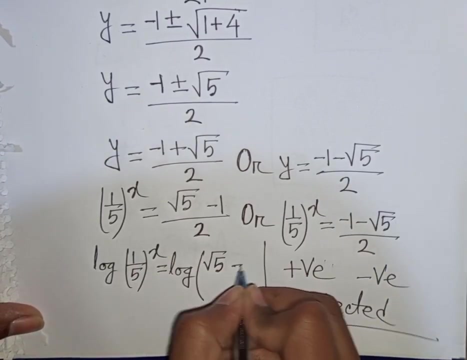 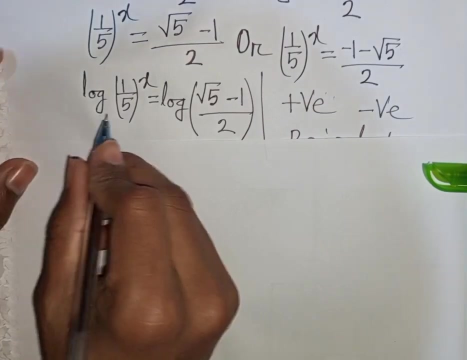 be negative, So positive cannot be equal to negative. So this is rejected. Now, from here we apply log in both sides, So you can write here: log of 1 by 5, bracket tau x is equal to log of square root of 5 minus 1 divided by 2.. Now, here you can apply. 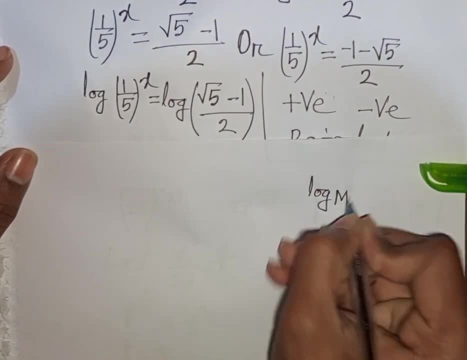 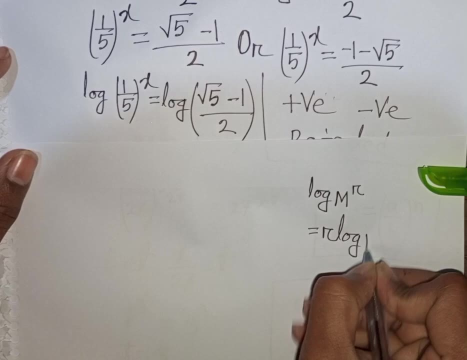 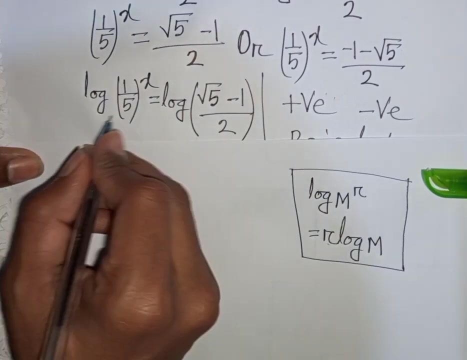 roll that log m. power r is equal to r log m. That means this power r move to the base. So according to this rule we can compare here- This power x will move to the base, So you can write. 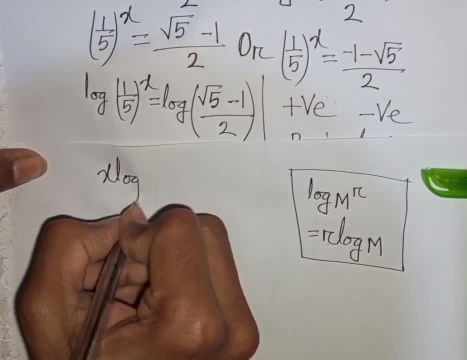 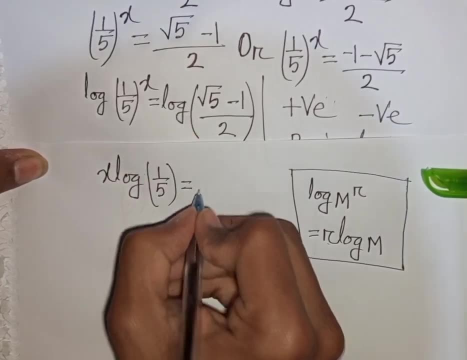 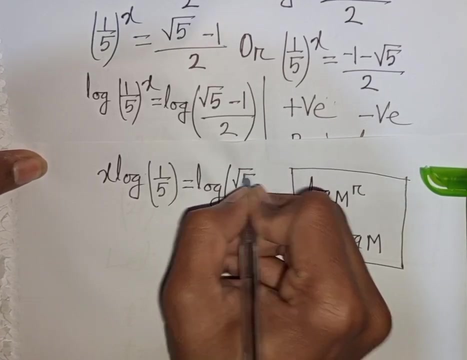 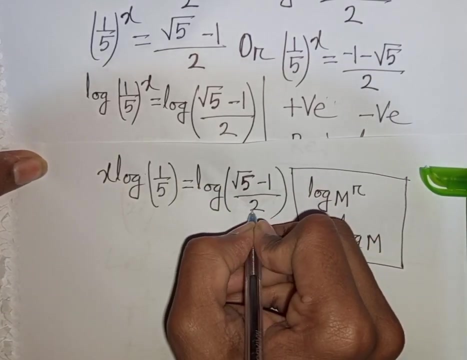 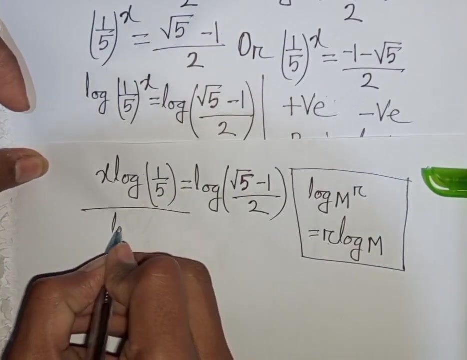 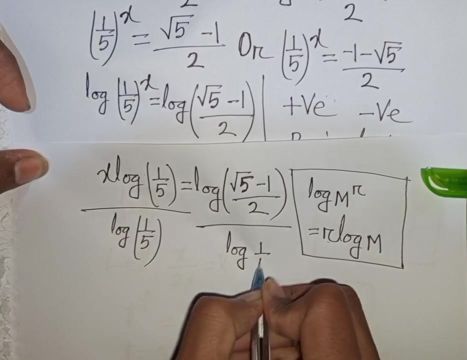 here, x log 1 by 5 is equal to log of square root of 5 minus on alpha 2.. Now we need the value of x, So we divide it by log of 1 by 5 in both sides. So divided by log of 1 by 5, divided by log of 1 by 5.. Now we see this log of 1 by 5,. 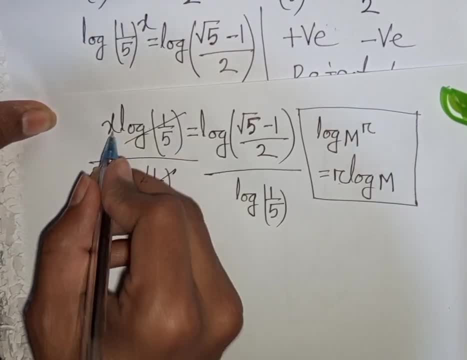 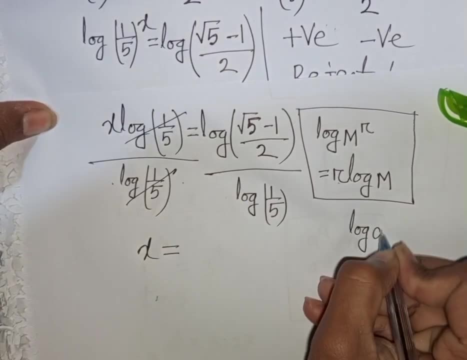 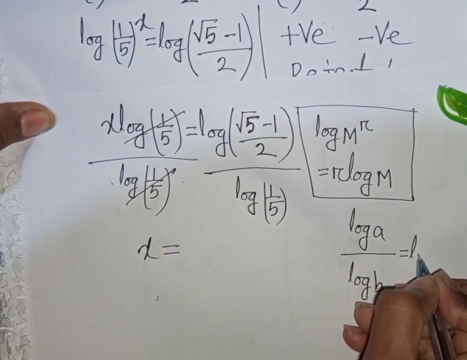 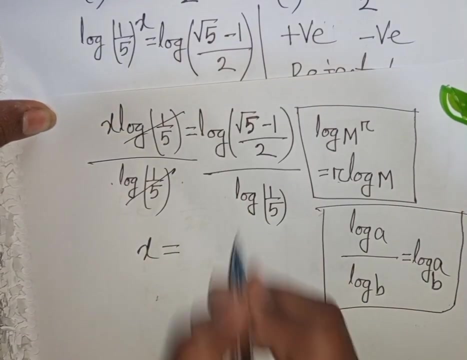 this log of 1 by 5 will be cancelled, So here x will be equal to. here I can apply this formula: log a divided by log b, This equal to log a base b. So according to this formula, this divided by this: that: 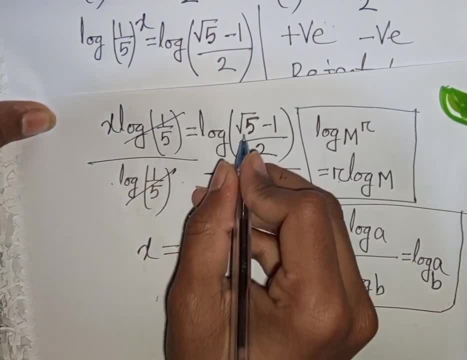 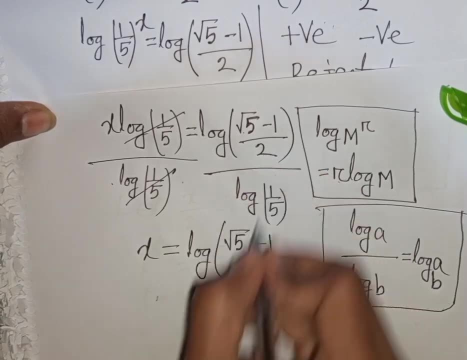 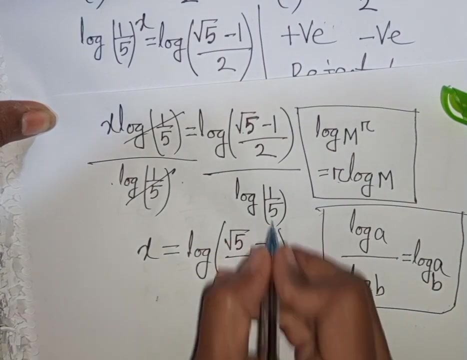 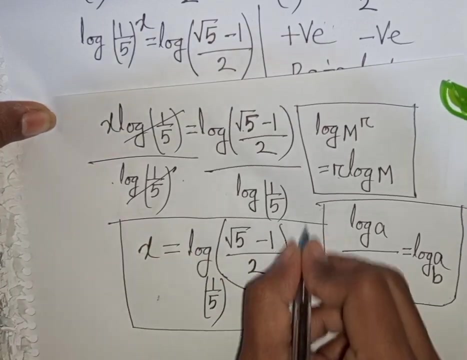 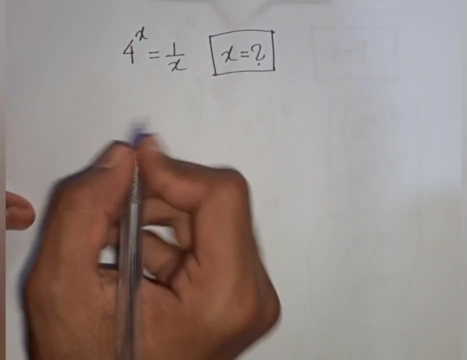 means it will be log of square root of 5 minus on alpha 2.. Then base of 1 by 5.. So this is the value. How to solve 4 power x is equal to 1 by x. Find the value of x. So we have 4 power x. 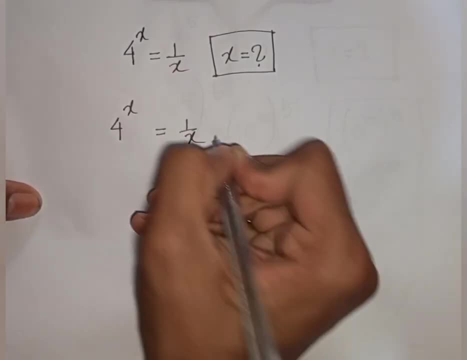 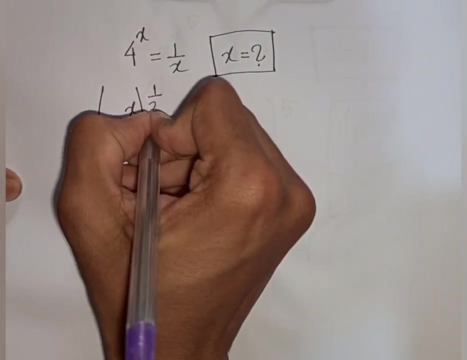 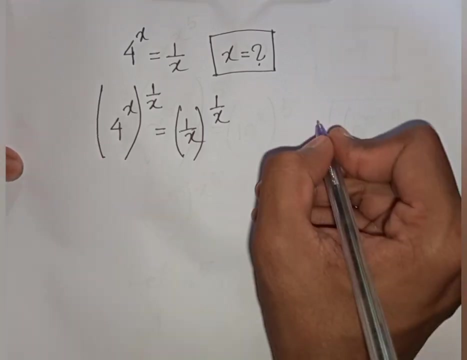 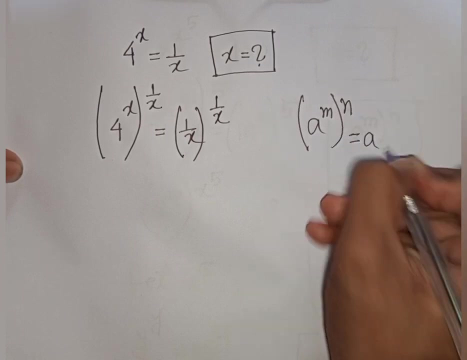 is equal to 1 by x. Now we multiply by power of 1 by x in both sides. So multiply by power of 1 by x, multiply by power of 1 by x. Now here you can apply this exponential that a power m bracket power n is equal to a power of m times n. That means 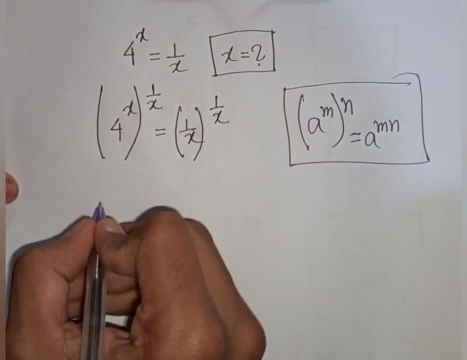 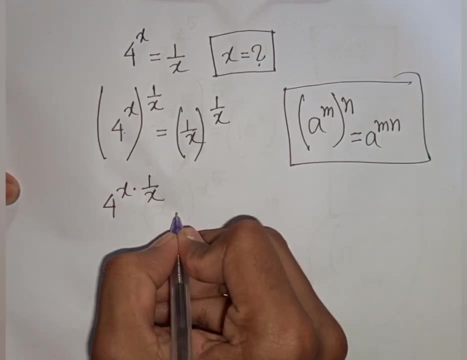 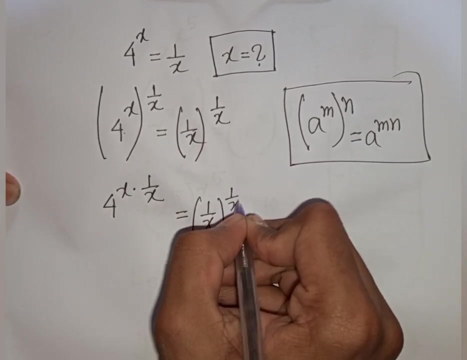 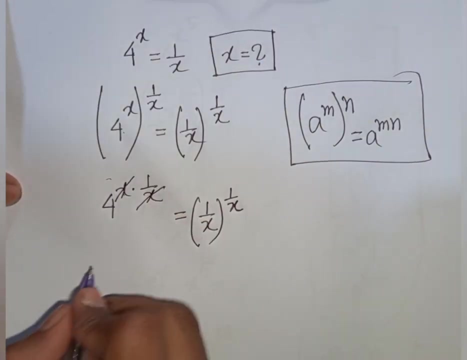 it will be mn. So 4 power of x times 1 by x then, is equal to 1 by x. So this is the power m. bracket power n. Now we see this x. this x will be cancelled, So we have. 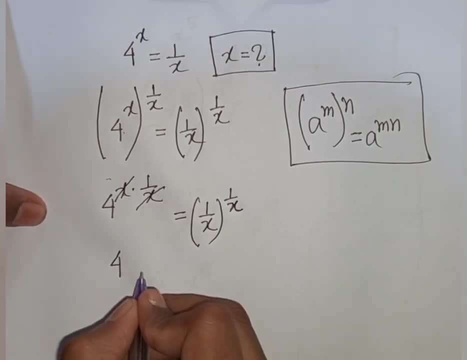 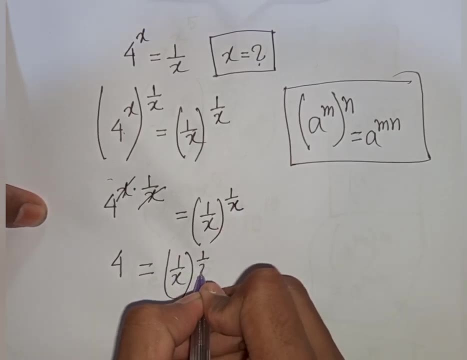 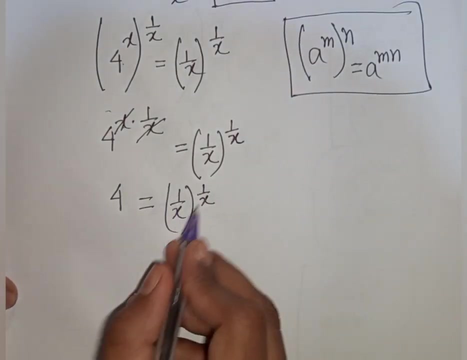 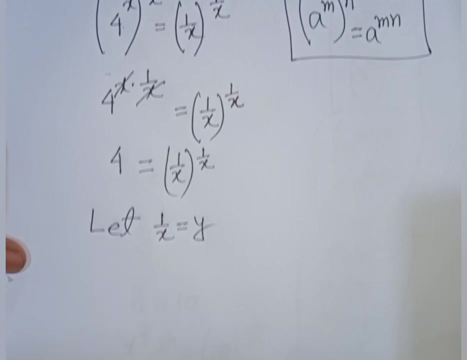 4. power n is same, as 4 is equal to 1 by x. bracket power of 1 by x. Now we see 1 by x, 1 by x. Base and power is same. So let 1 by x is substituted by y. So our equation: 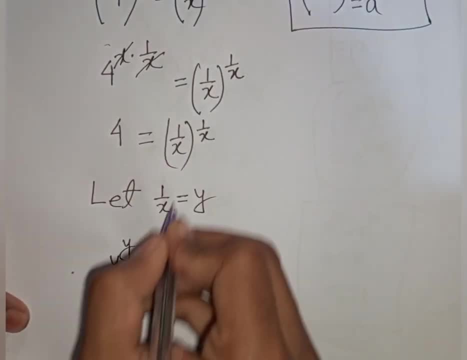 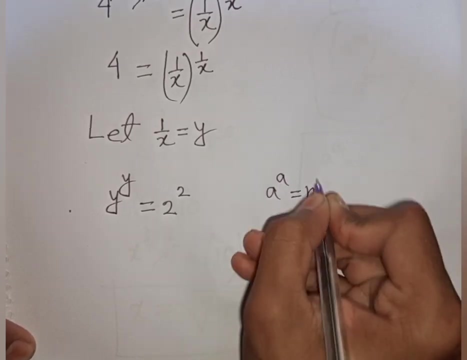 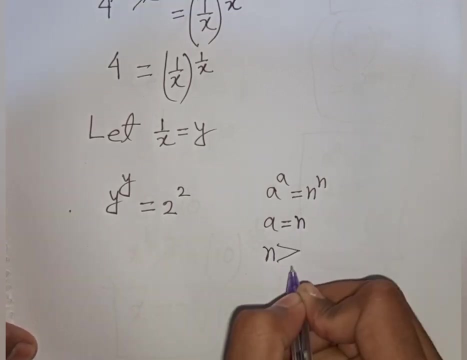 will be y power y is equal to 4.. So 4 is same as 2 power 2.. Now here you can apply rule that a power a is equal to n power n. So a will be equal to n. Oh yeah, n is greater than or equal to 1.. So according to this rule, we can compare. 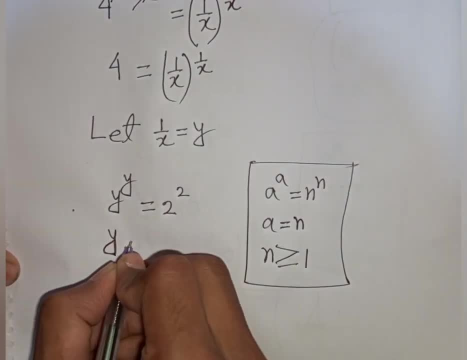 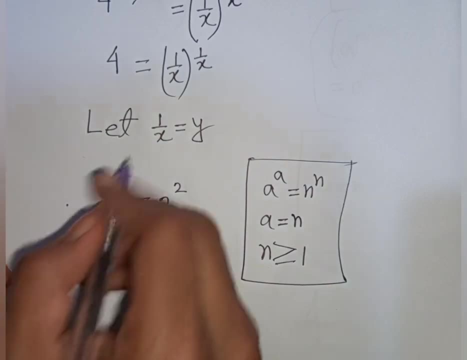 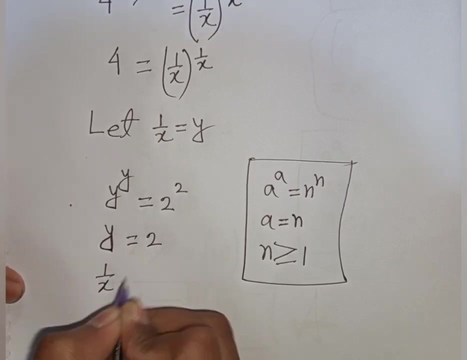 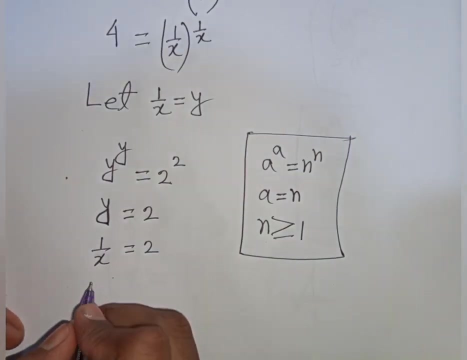 here y will be equal to 2.. But remember that 1 by x is substituted by y, So y, that means it will be 1 by x, is equal to 2.. Now here you can apply cross multiply, So you can write here: x times 2, that means it will be 2x is equal to here, 2 is same. 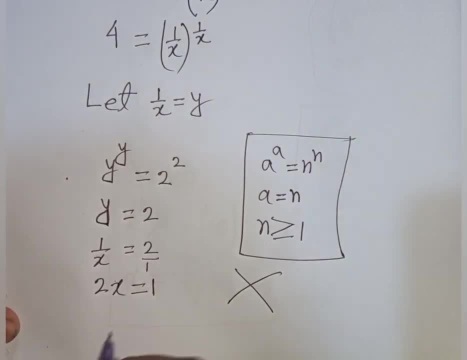 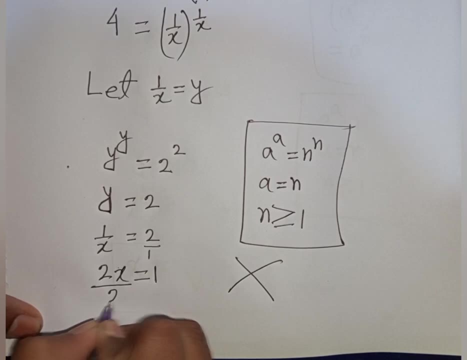 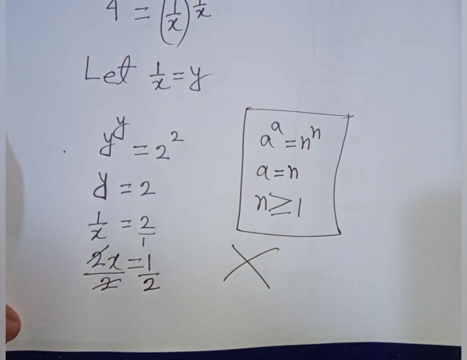 as 2 by 1.. So 1 times 1, that means it will be 1.. Now we divide it by 2 in both sides, because we need the value of x. So divided by 2, divided by 2.. Now this 2, this 2 will be cancelled. So we have x. 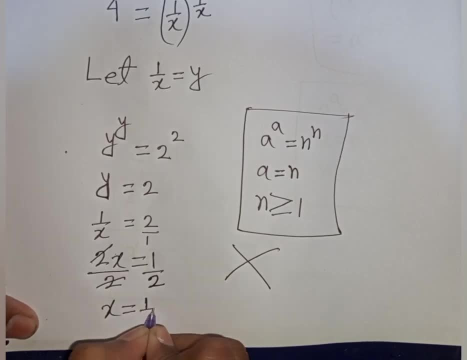 is equal to 1 by 2.. So, 1 by 2, this is the value of x. So this is our final answer.